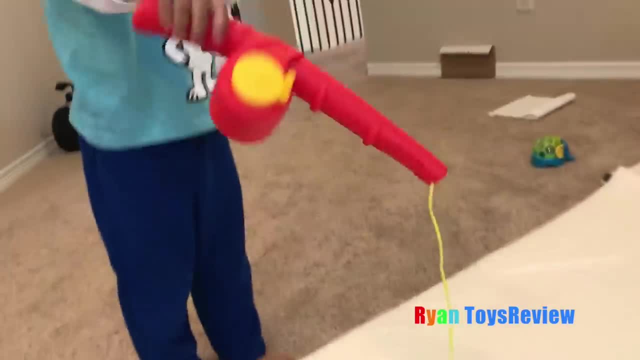 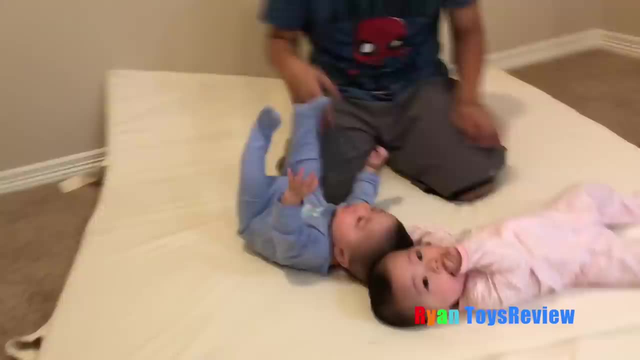 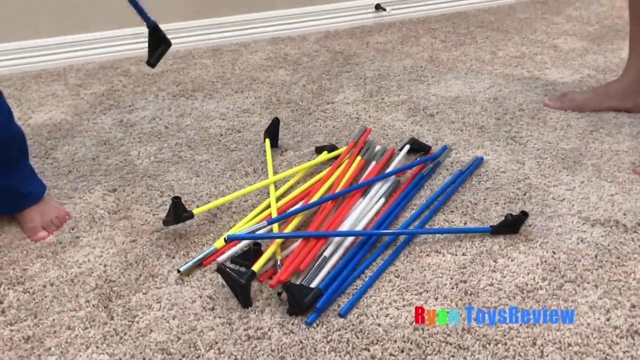 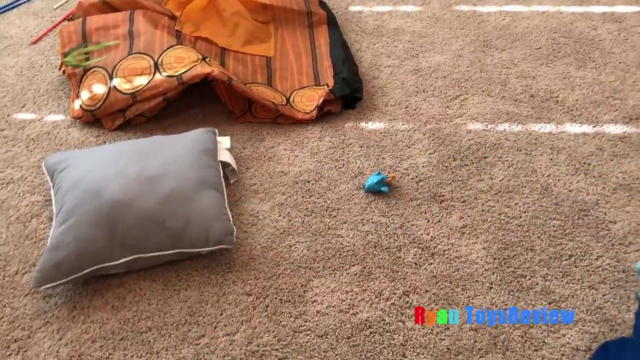 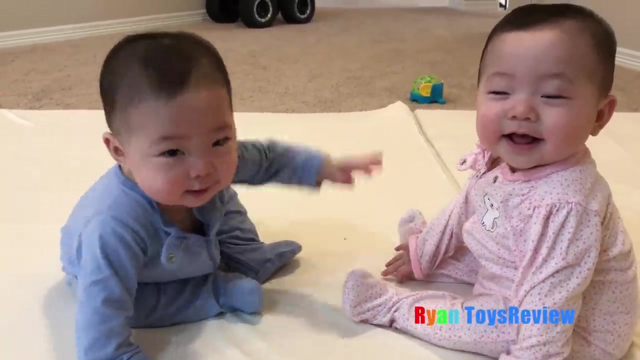 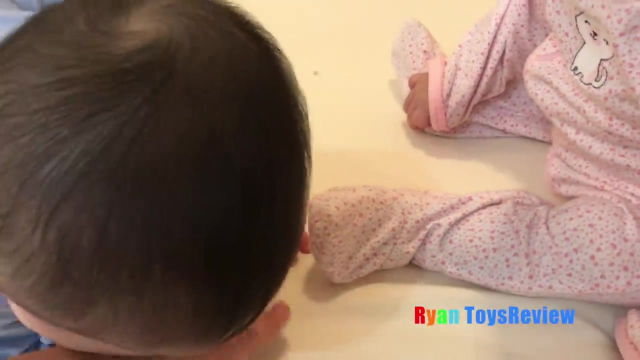 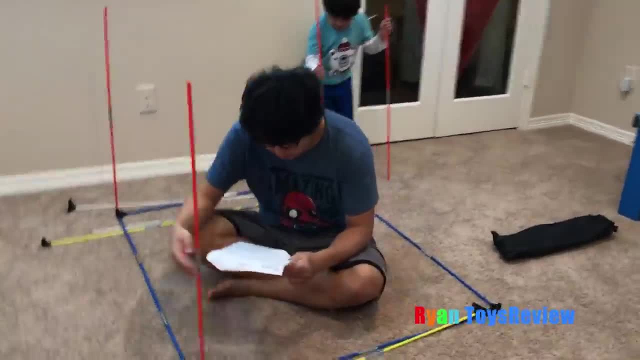 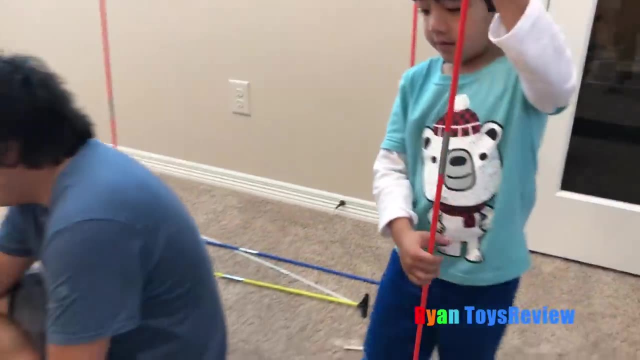 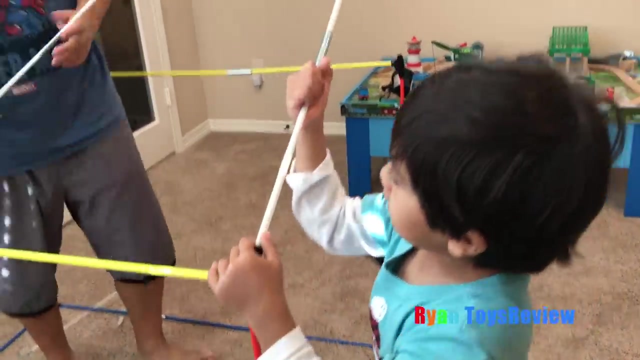 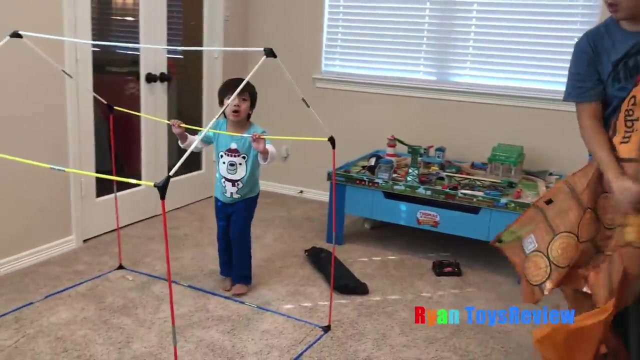 Kids. this is what it looks like It's going to be looking like in the inside. Oh wow, It's like a practice to build a real tent, Got it? You know what to do. You know this, Harry. Oh, this is a very shaky tent. Oh, this looks like a barn tent. Oh yeah, it does Not just like a tent, it's a barn too. 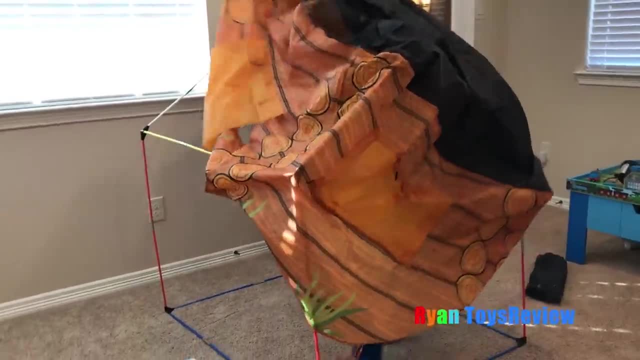 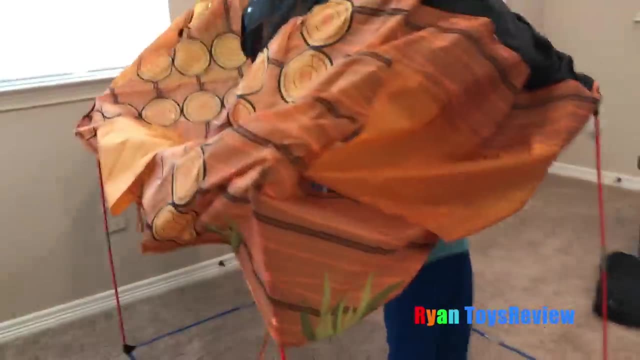 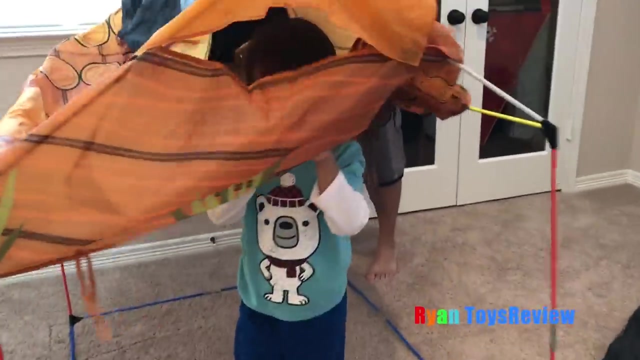 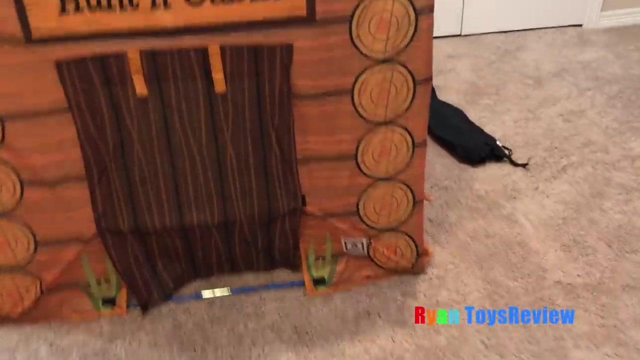 I'm already going to go in here. Oh no, where's Ryan? Are you trapped inside, Ryan? you're trapped inside the tent, here Into the cabin tent. Ah, there he is. I can't see your head, That's right, I can't see my face. Where'd you go? Ah, Okay, where's Ryan? I see a hand sticking out of the cabin. 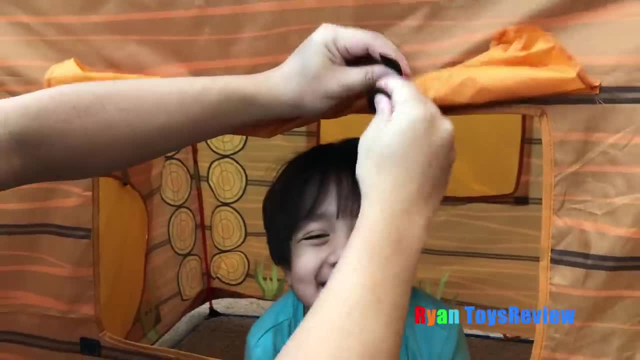 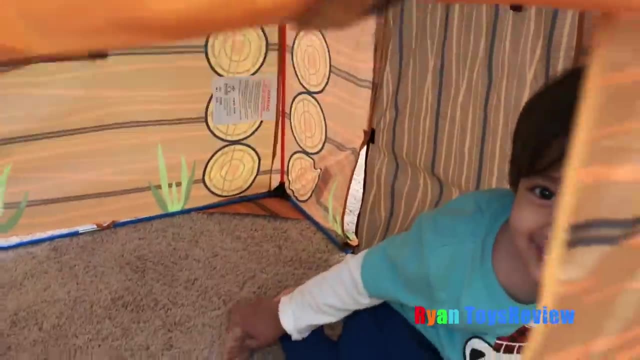 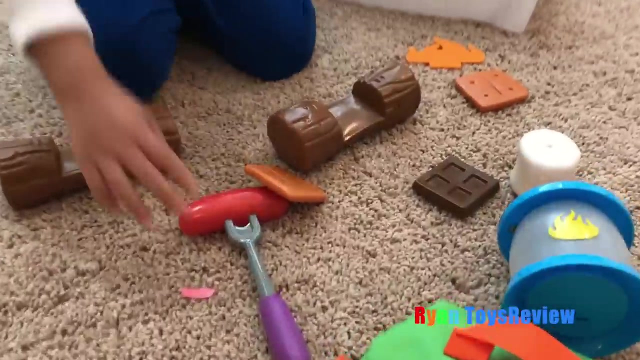 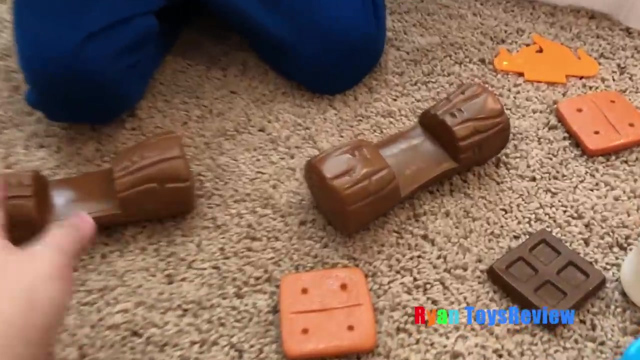 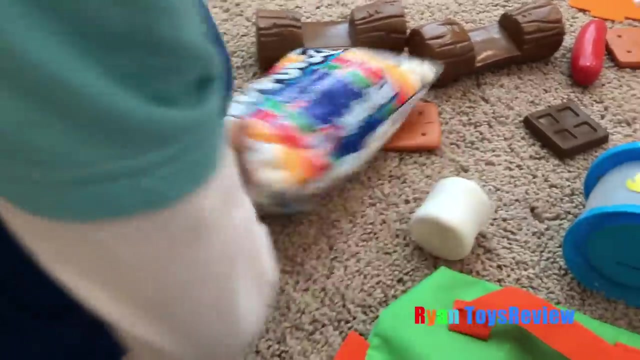 Woo hoo, Hi Bye. Ah, where'd your brother go? Ah, see you, Look there's a campfire. Ah, Oh, so what's included here? I thought, why do they put a hot dog? Yeah, people like to eat hot dogs in the campfire. And here's some logs And we also have a marshmallow. And we also came with a big marshmallow, A little one. 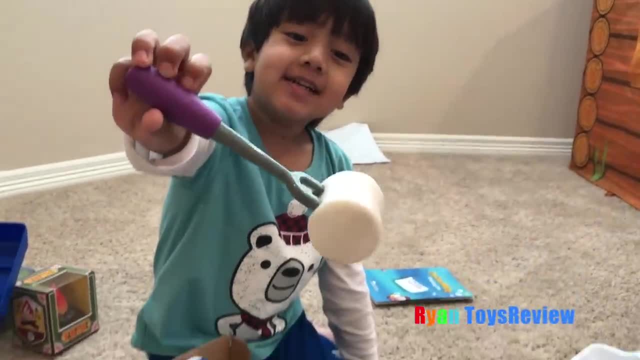 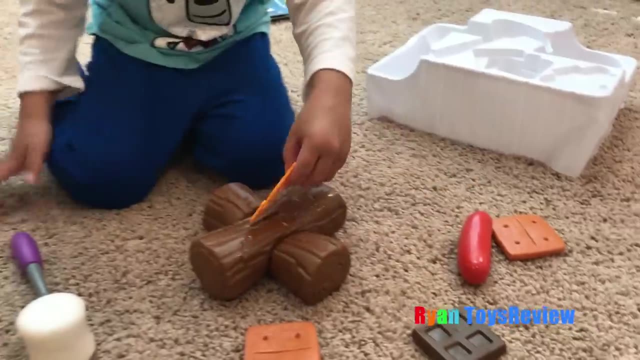 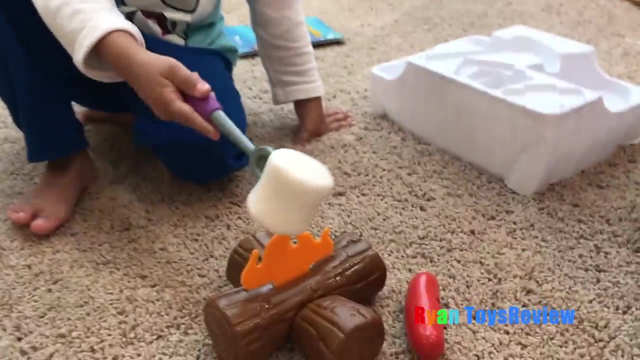 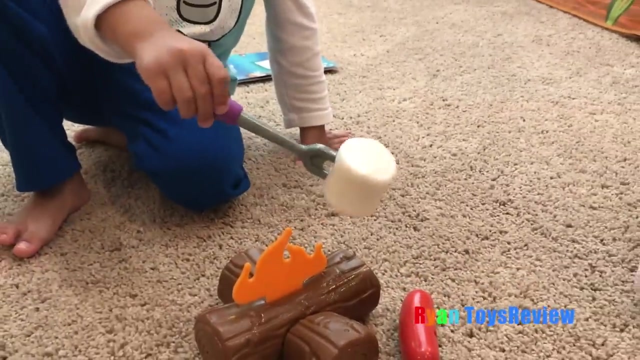 Hmm, Looks like Okay. and then the fire goes there. That's right. Ah, All right, don't catch the fire. It's hot, Okay. so Ryan's going to roast some marshmallows. Ah, I burned it. Don't burn the marshmallow, You're going to rot, is it? Yeah, There you go. 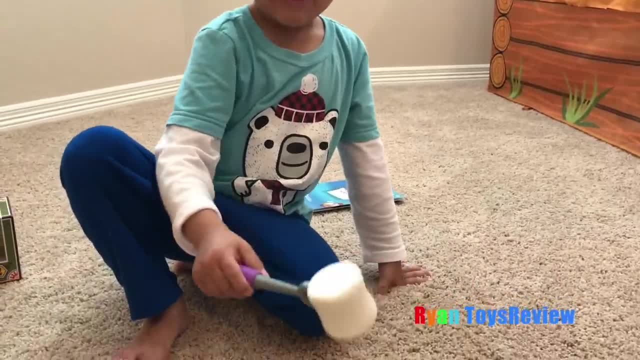 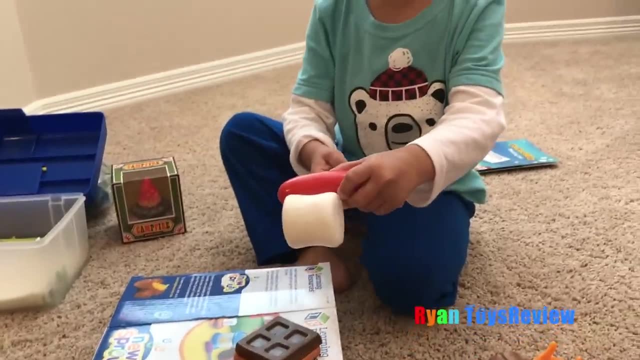 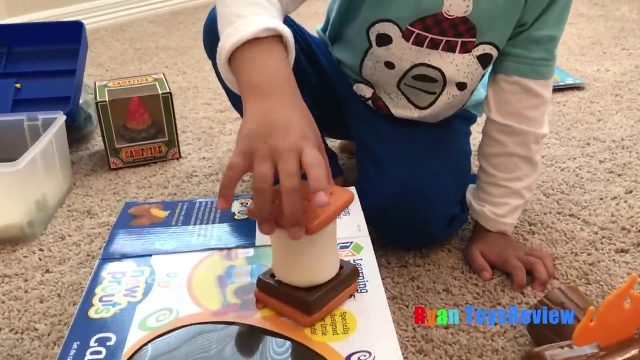 Ah, I think it's done. We have a chocolate piece And some crackers. Wait, you didn't. You're using sausage to kick it out. It's hot, It's hot. There you go. That's it, Ah. 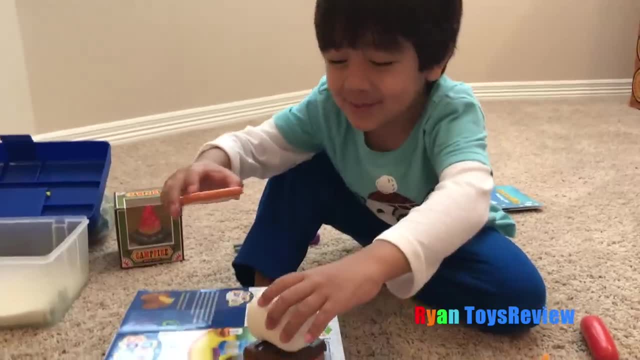 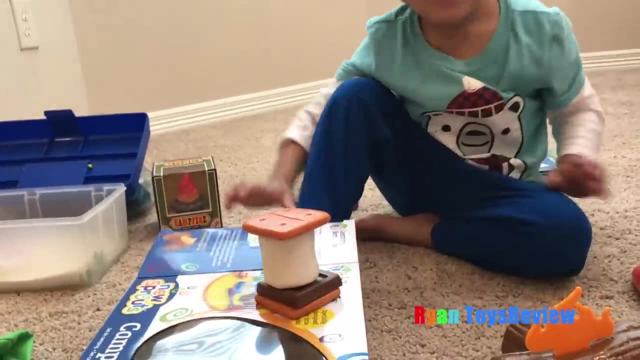 One thicker, Because if I do it this way it's going to roll off. Oh yeah, that's true. Never seen this more that thick. Wow, it's huge. Who's going to try to eat that? Oh, oh. 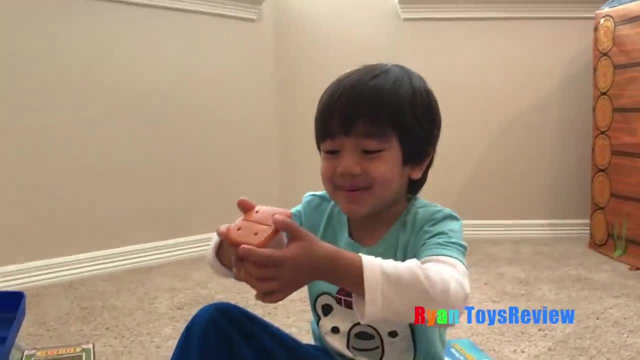 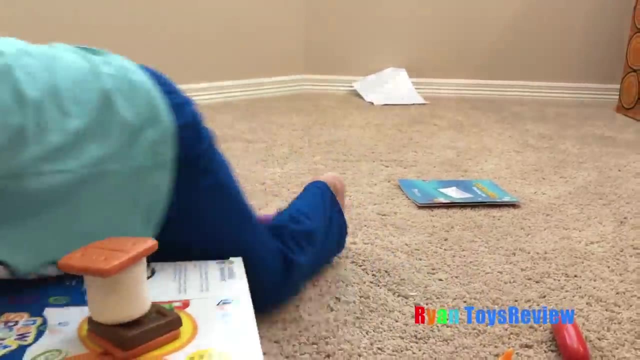 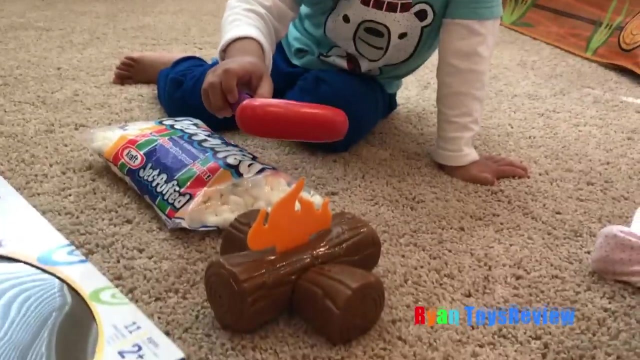 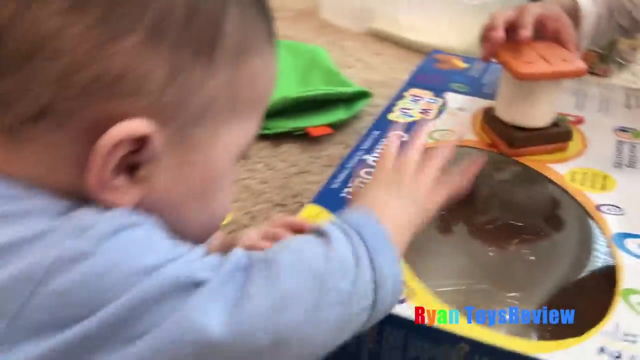 Ha, It's even bigger than my mouth, That's true. That's so huge, That's funny. It's time for some sausage. Ah, Hey, What's going on there? Here's some big- Oh sorry, Ah- veggie sauce. 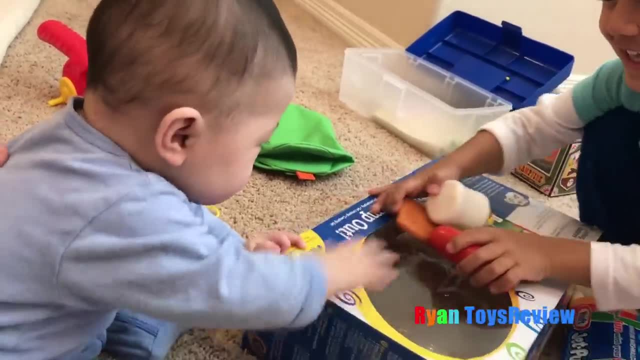 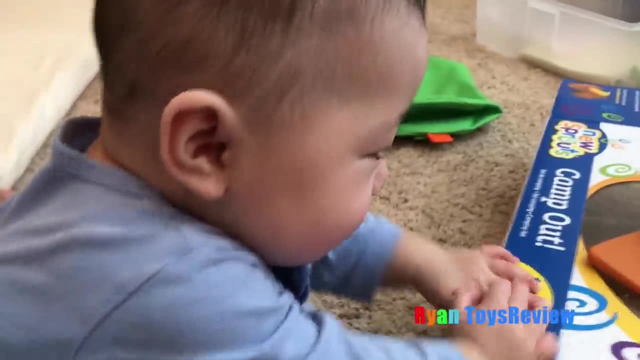 She's like: I want, I want some too, you guys? Oh, thank you, Is it yummy, Yummy? I think she wants some, She likes it, She likes eating these. Yeah, And we're going to try these mini marshmallows, because Mommy forgot to buy the big ones. 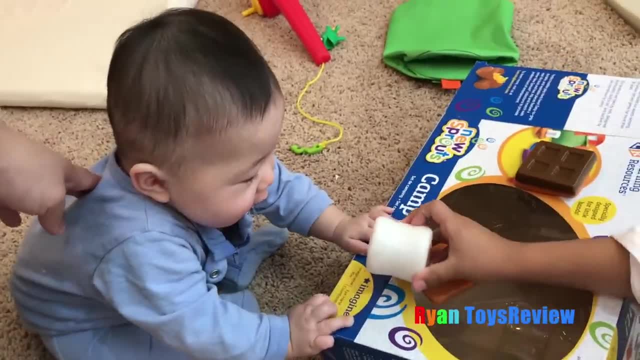 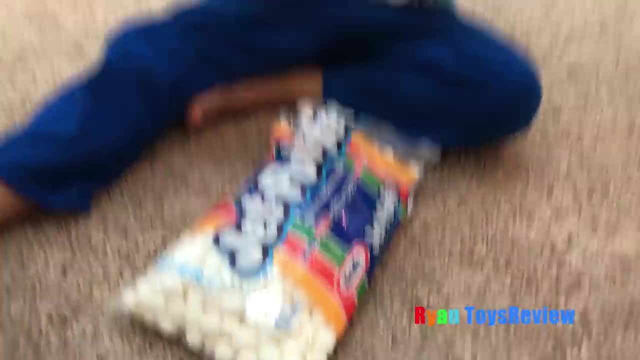 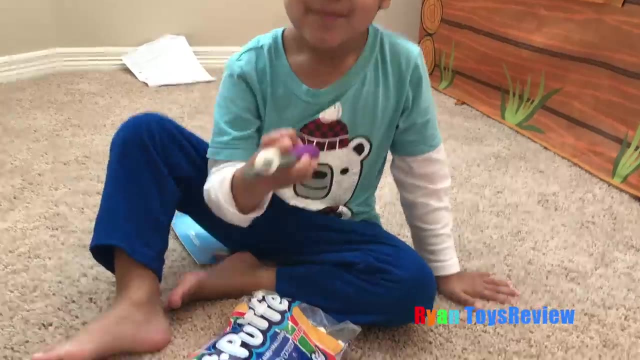 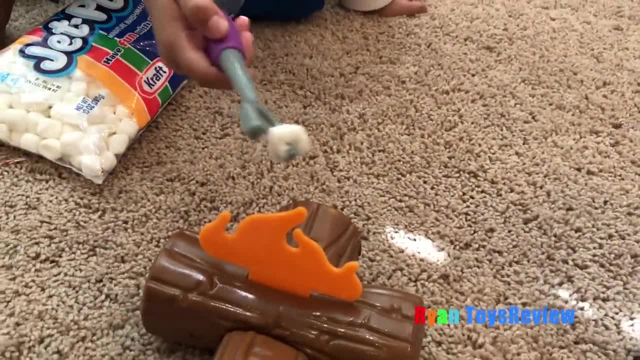 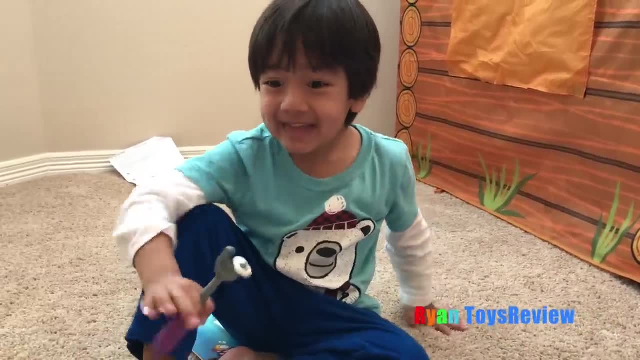 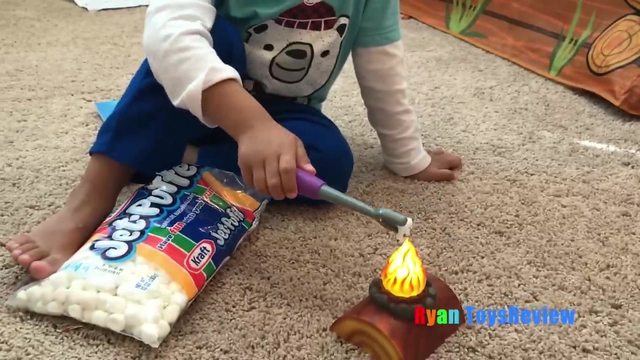 Oh, Oh, Oh, Oh, Oh, Oh Oh, Ori gelen Yummy marshmallow, Yummy Yummy in your tummy. So we got a Night Light version, Whoa, And it lights up like a campfire. 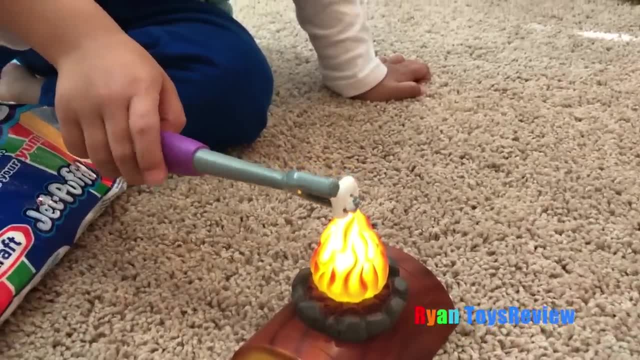 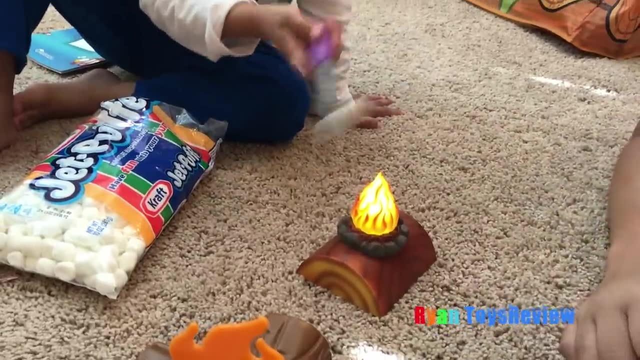 Rose of marshmallows. Are you doing the real marshmallow? Yeah, You got to rotate it right. Or is it going to be burnt? Oh, see This. Yes, I want some. You want some marshmallow, Emma. 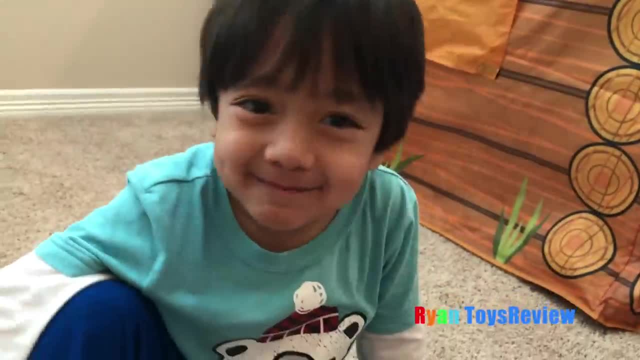 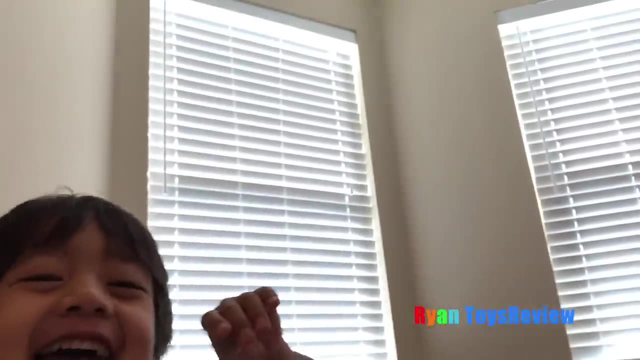 Hi, Hi, Time to go fishing. The first fish is you. What? The first fish is me? I didn't expect that. Oh no, Some fish on the floor, Whoa. Oh, nice Water came off, Yea. 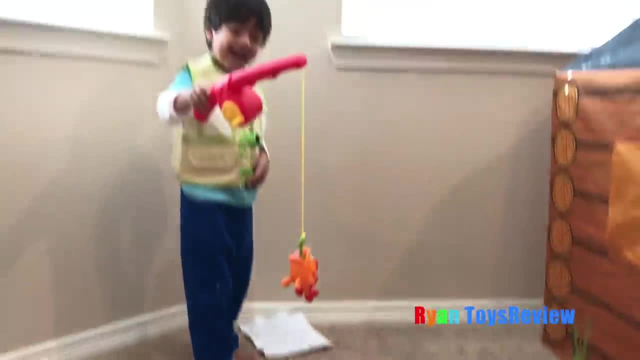 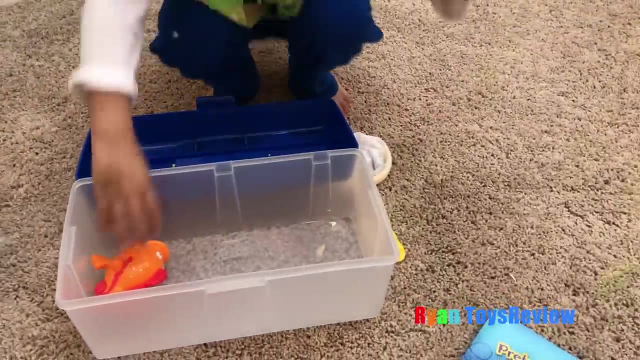 He ate the worm. There you go. He ate the worm, He ate the worm. I need another worm, You need another worm. I want a worm. I want a worm, It's a worm, It's a worm. Look. 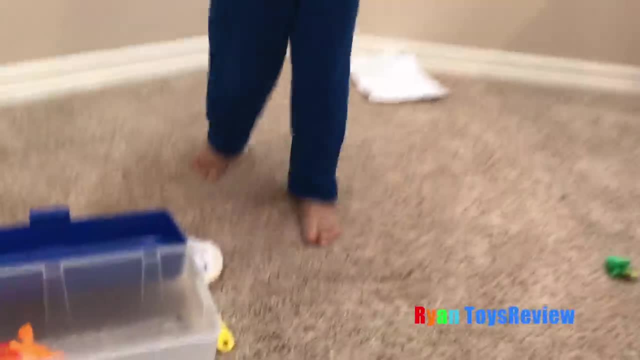 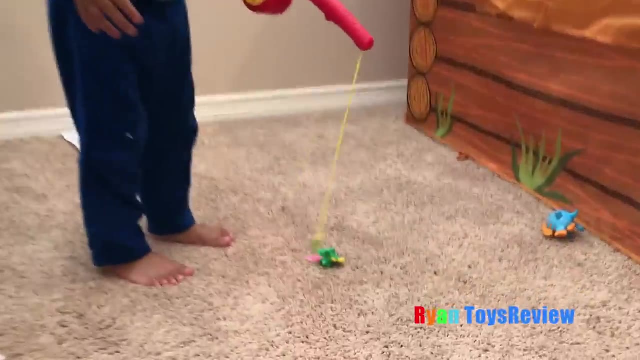 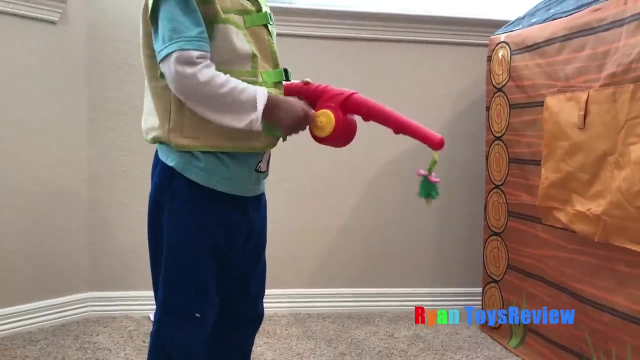 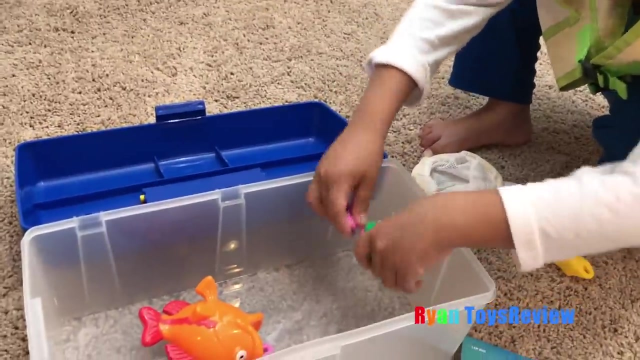 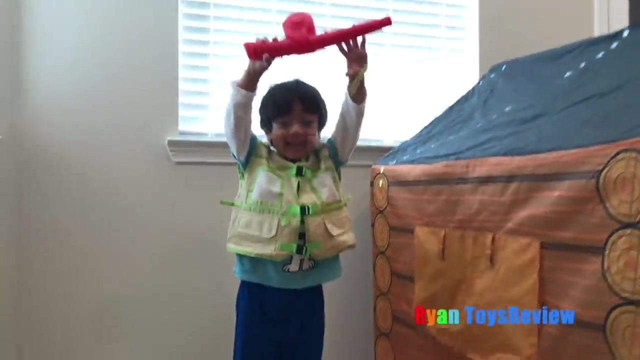 I want a worm. It's a worm. I want a worm, I want a worm, I want a worm. another warm, There it is. You got it. Oh, there's two other warms. Time for another fish. Can you get it Too hard with the warm? Oh, you got it Nice. Oh, no, it's warm. Aw, you got it. Oh, nice, You got it. I got it. Oh, I fell out. 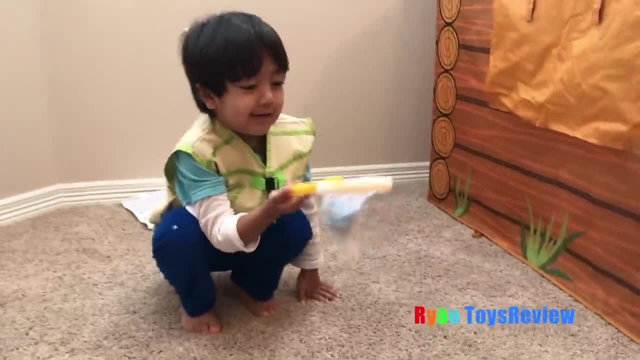 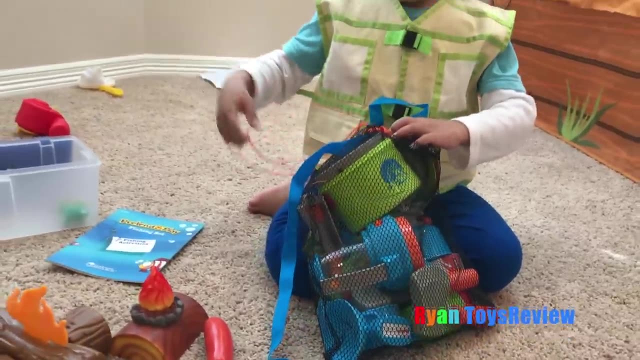 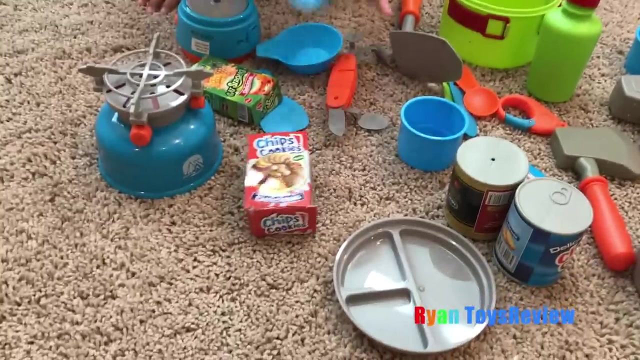 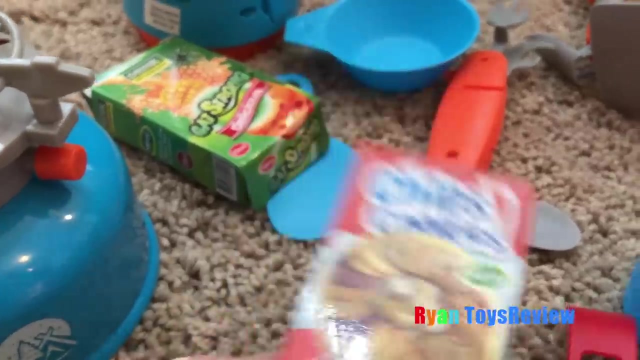 Gotcha Cool. So we also got some other camping gear. Let's see what's inside. It's a survival camp, Survival camping. Yeah, let's see. Here's what it comes with. Oh, looks like you can add some ingredients in here. Oh yeah, And it comes with some chip cookies, But there's. 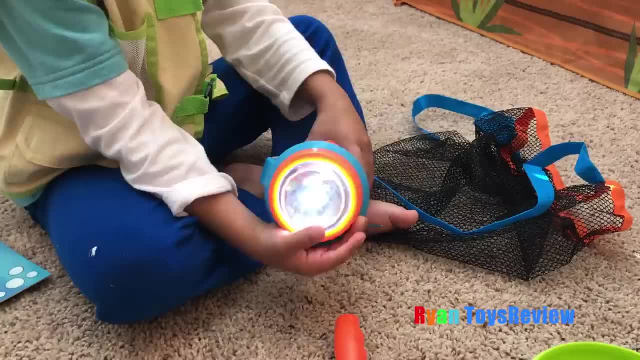 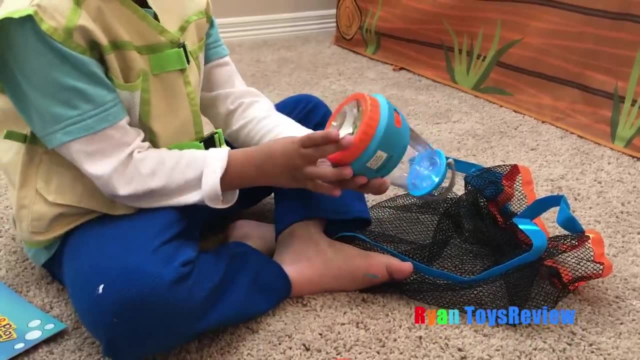 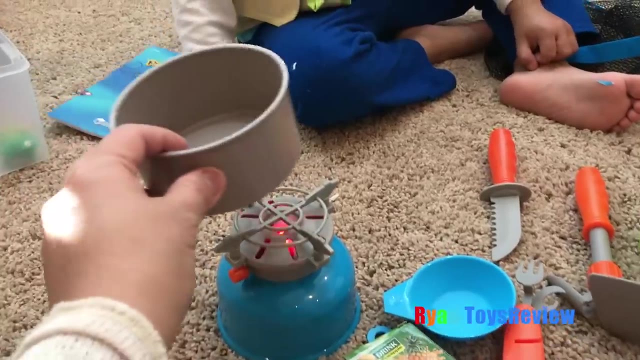 no chip cookies. Yeah, and a drink. Look This side. when you're doing this side, the back lights up. When you do this side, this lights up. Oh, I see, That's cool. Yeah, so that's where you put the food. So you put. 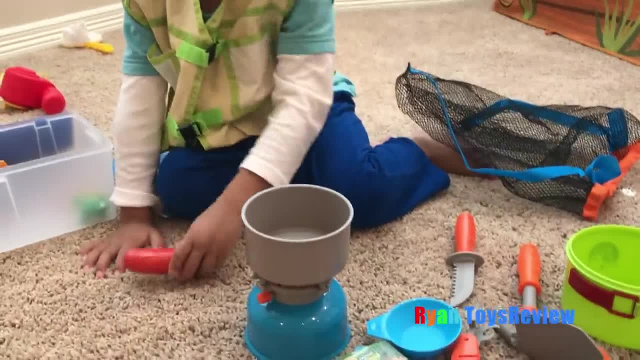 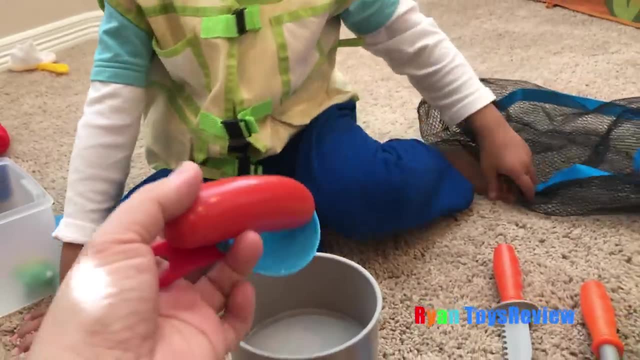 food there, like that, and then you pick it: Sausage. Yeah, Oh, there you go. Okay, let's scoop it out. Let's see, Ah, you're touching the bowl. That's not right. Scoop it out and. 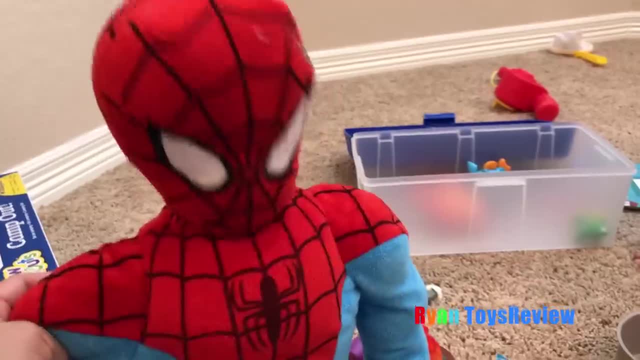 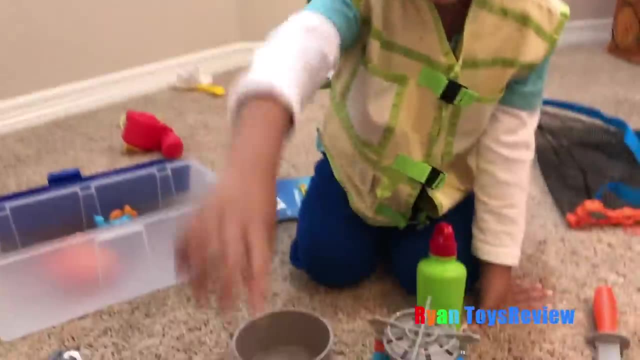 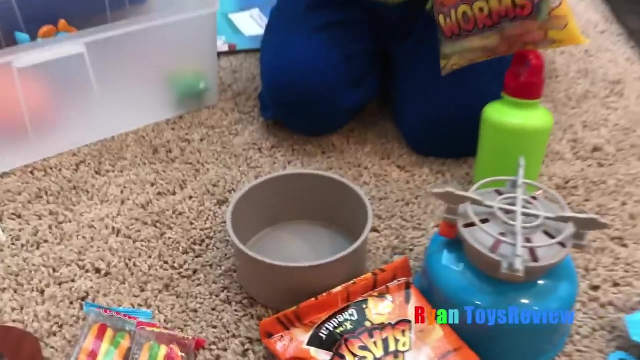 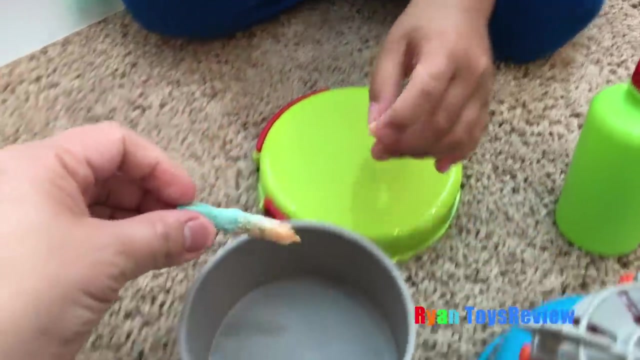 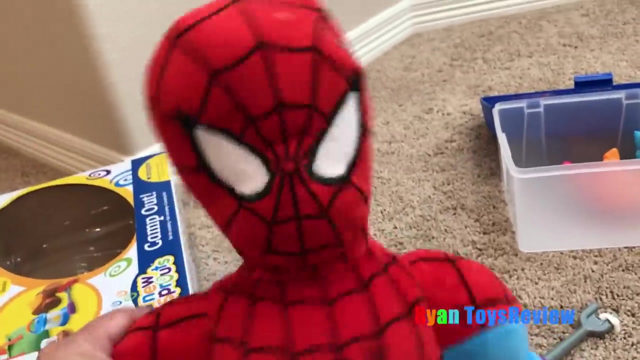 put it on the plate. Hey, Ryan, Hi, I'm hungry. Can you please cook some food for me? I want something sour. Oh, how about this? Oh yeah, Some Warhead Worm. That sounds good. Oh, is this going to be gummy soup? 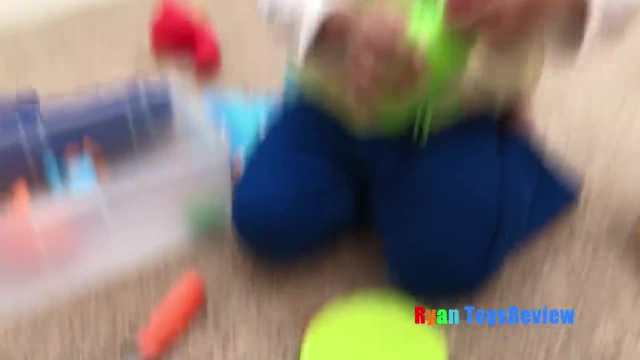 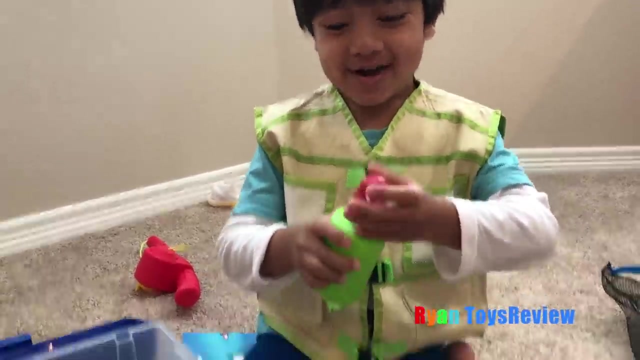 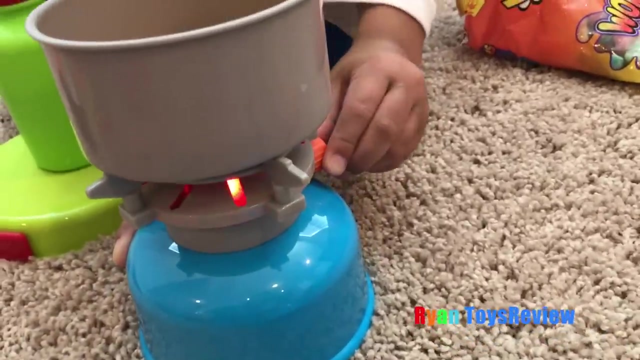 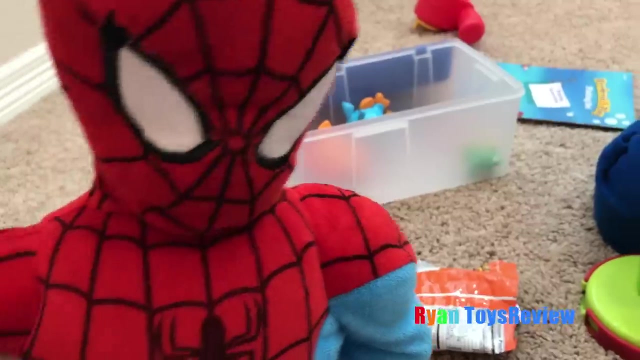 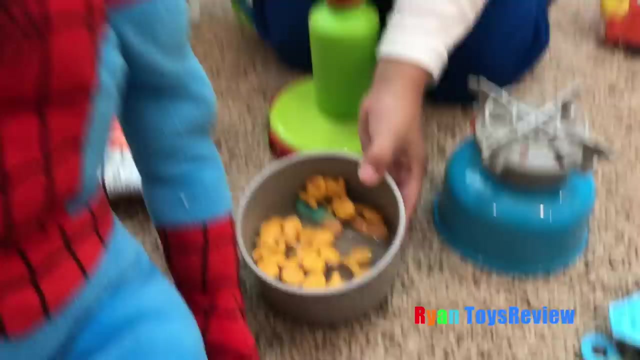 It looks like gummy soup. It's sour water. Oh, It's water, but it's sour. I see, Ooh, goldfish, that's my favorite. Ooh, smells delicious. Is it ready? Oh nice. 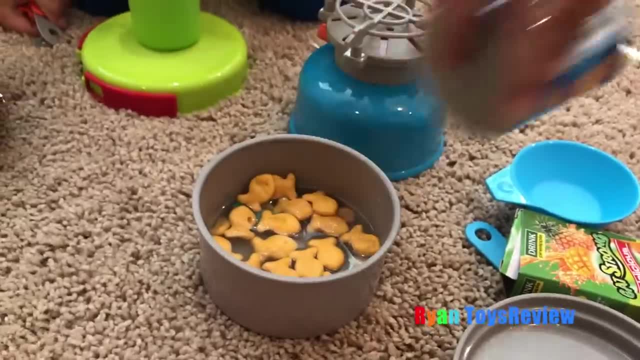 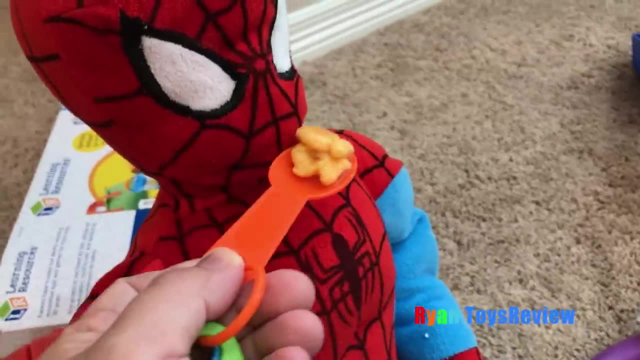 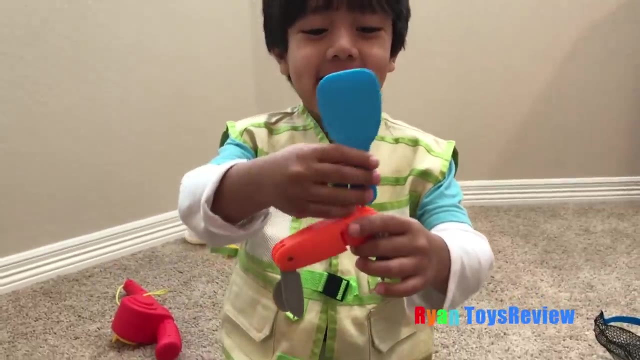 Open it down. Whoa, thank you. All right, some goldfish for you. Spidey, There you go. What do you think That was delicious? Thank you, Ryan. A doggie That looks like a doggie. 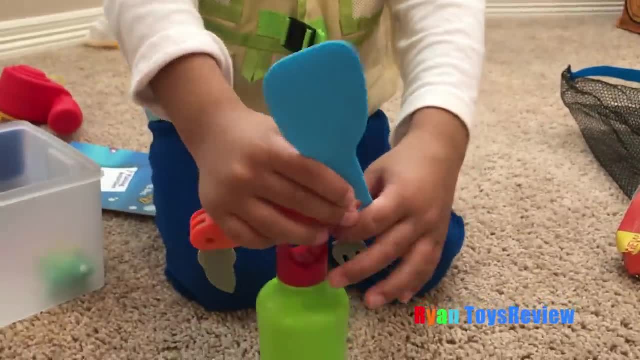 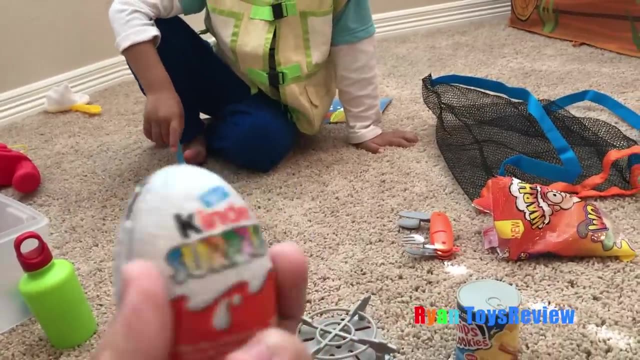 Cool. Aw, Muff, muff, muff, muff. Mommy, are you going to cook something for me? Yeah, I'll cook something for you. Okay, are you ready? I got some Kinder Surprise eggs. They're going to go in here. 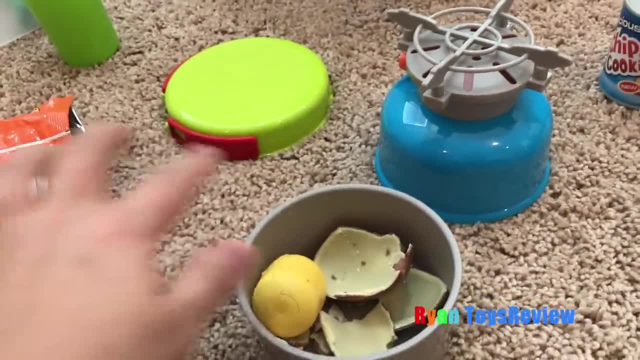 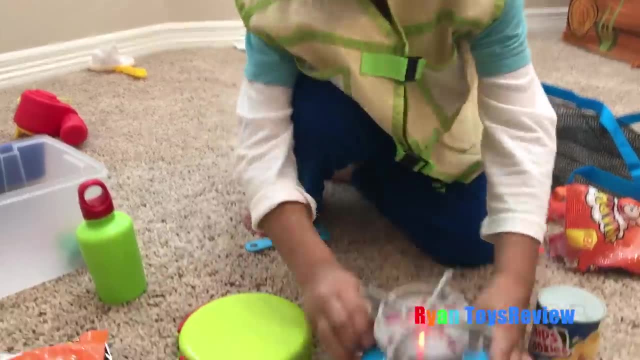 If you put it on the stove, I'm going to flip it. Okay, It comes with the surprise toys. We can't cook this, It's going to just go up there. Okay, Thank you, And then I'm going to put in some gummy hot dogs. 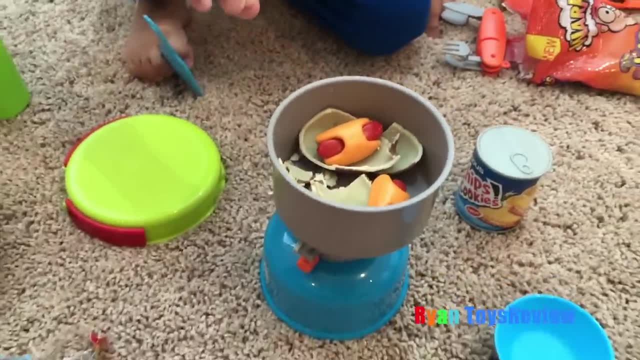 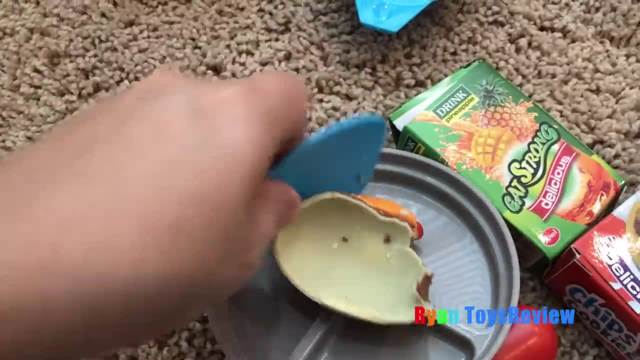 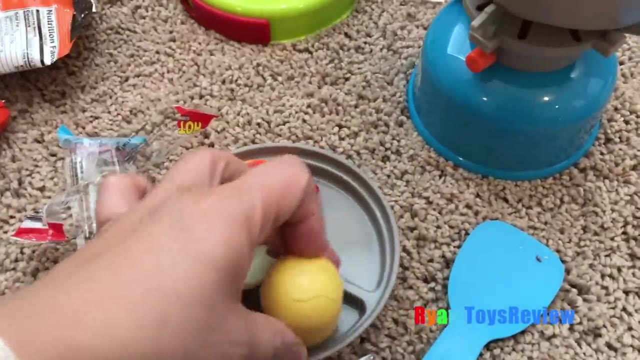 All right, some gummy Hot dog goes in there. Okay, let's stir it for Ryan Too hard. Okay, put it on the plate. There you go. There you go, Mr Ryan. Oh wait, And a surprise toys from the Kinder Egg Surprise. 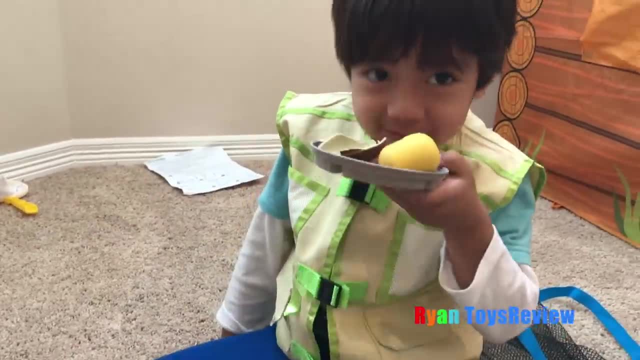 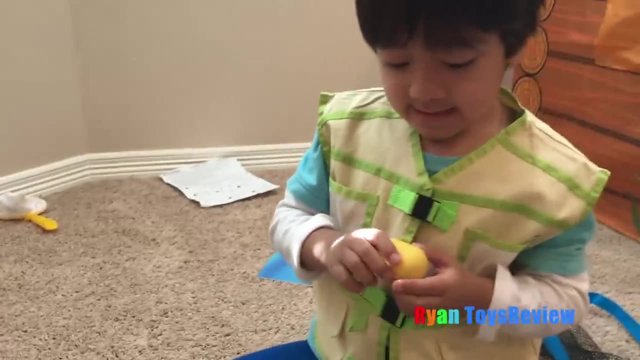 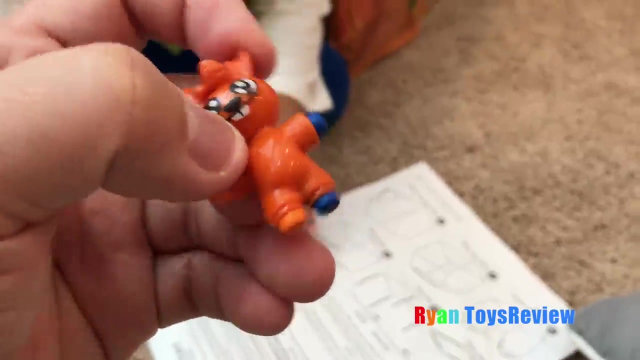 After I'm done. That's right, Here you go. I ate all. Now I can do this Kinder, Yeah, so Ryan finishes food. What did we get? Got a cute thing, Something cute, This toy. it's like a crayon. 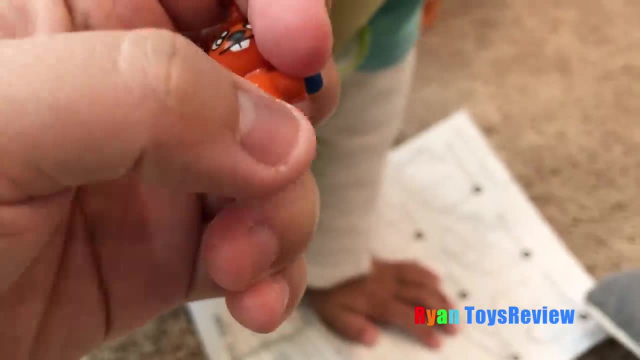 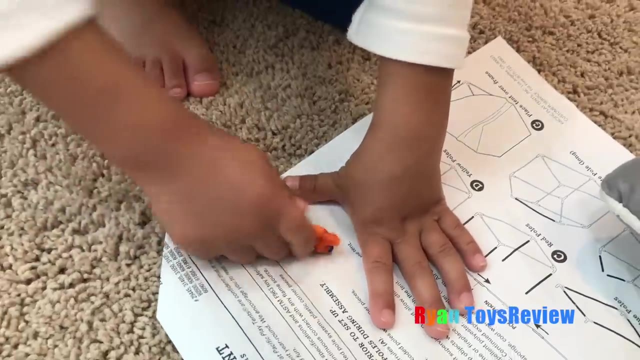 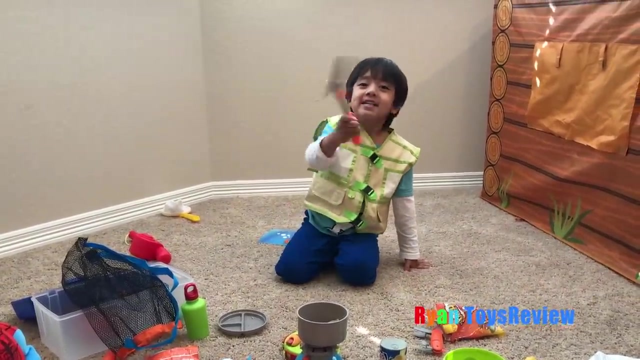 You can draw blue from the hand and one of the feet, and also orange, So it comes with blue and orange colors- The hands too, It's true. Thank you, guys for joining me on my camping trip. Bye, Bye- Spider-Man also says bye. 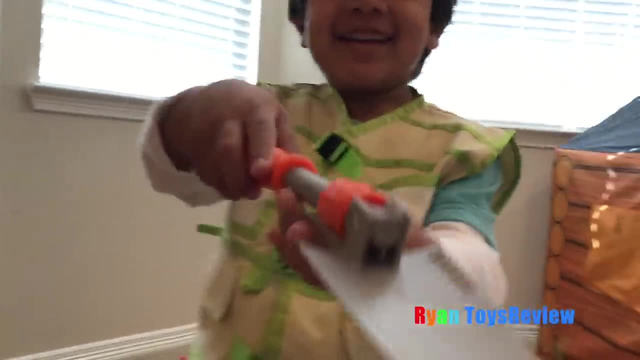 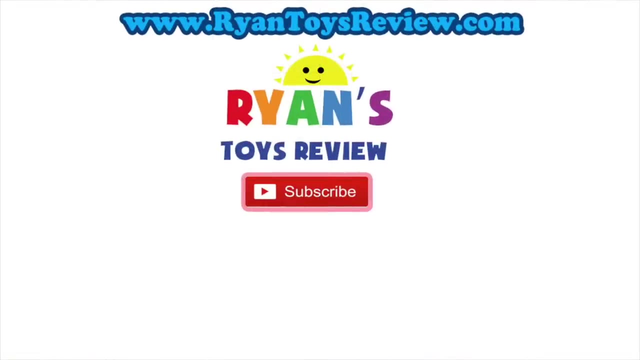 Bye, I'm going to pick you up as well. That's dirt. Oh no, I'm dirt. I'm dirt. The phone is big. Please click on one of these videos for Ryan Toy Room and more fun.